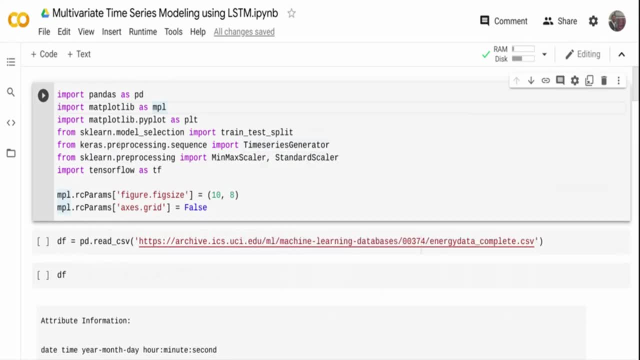 data preparation of time series model. So it's in the Keras preprocessing package and I'm importing time series generator From the sklearn preprocessing package. I am importing standard scalar and minmax scalar. I'm using only one of it, but I will tell you like why I'm using. 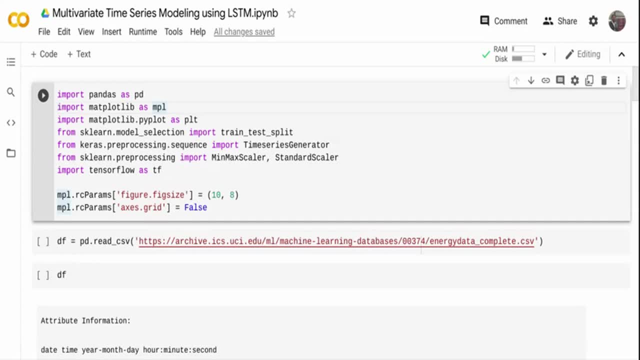 the necessary scalar, And then I'm importing TensorFlow to define our LSTM architecture. So that's what I'm importing. So once I have this, I'm going to download my data set. My data set is in the UCI machine learning library- open data set. So I'm going to use the energy data. 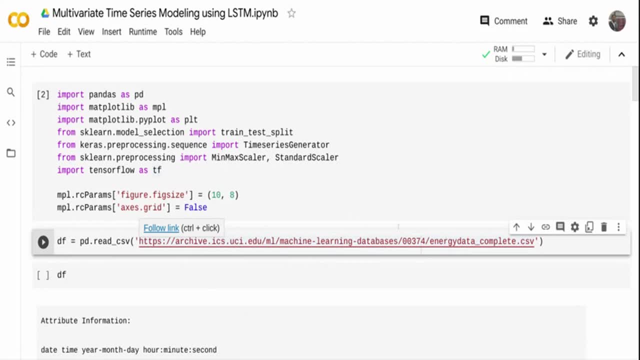 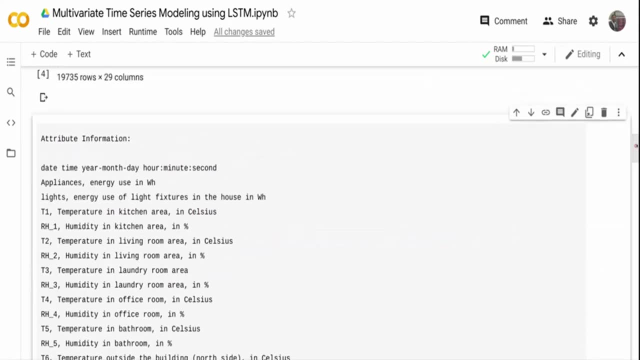 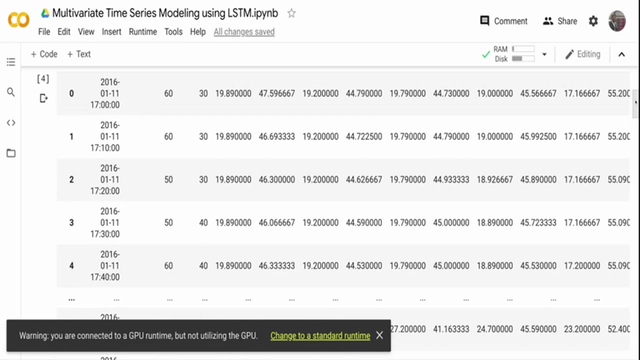 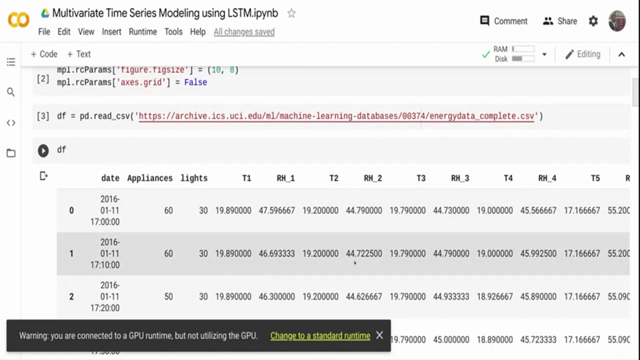 from that particular UCI library and I'm assigning it to a data frame. So once I download the data and run it, you can basically see there are like close to 19,735 rows and 29 columns. So you can see. over here on the top you have all the date: appliance light, the energy usage for the appliances, the energy usage for the light. 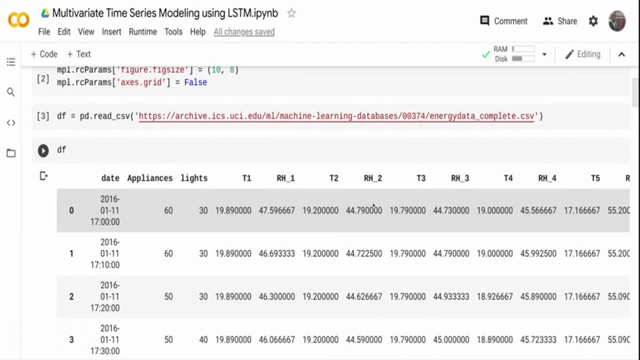 And then there are a lot of T1, RH1 and T2, RH2.. I will tell what are these columns. So the date. if you see, we have data collected every 10 minutes. So basically, these are like smart meters that are fitted into an house. 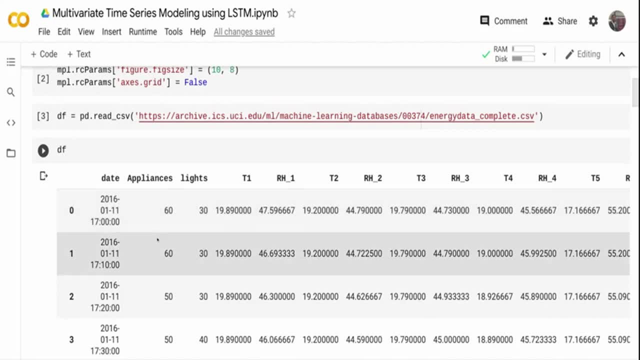 And the data is collected every 10 minutes, which tells us the appliance energy usage and the lights energy usage, And there are a lot of other parameters like temperature. All this, T1 is temperature and RH1 is humidity. So I have defined the columns below. 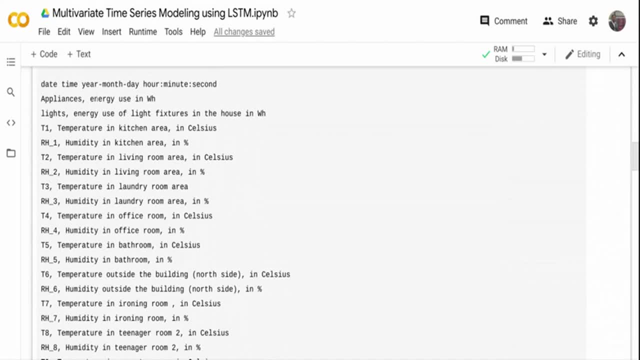 I have taken it from UCI and pasted here. So the appliance is basically nothing but an energy usage in watts And the lights is energy usage of light in watts. So when I say appliances, these are like heavy appliances, like your washing machine or even like heater, AC and all. 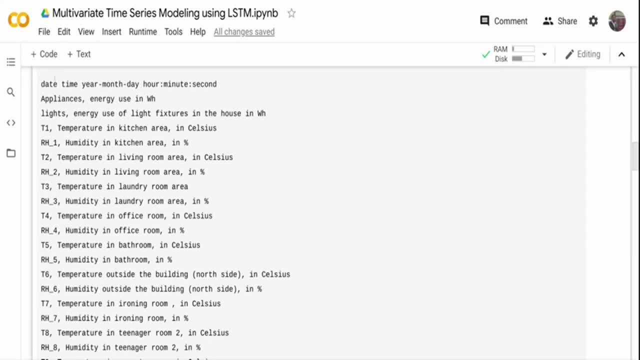 Lights are general lighting that you use in the house. The date is the time, Which is every 10 minutes. the data is captured And I have like temperature and humidity for each and every room in the house. So I have the kitchen area temperature, kitchen area humidity. 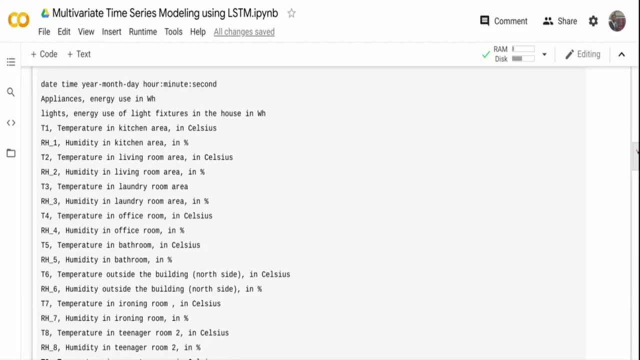 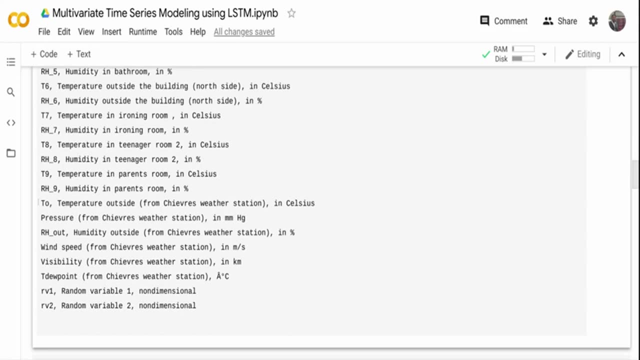 I have the living room temperature, living room humidity. Similarly, for each and every room in the house, the temperature and humidity is captured. Apart from that, there are variables that capture outside temperature Like TO stands for temperature outside and pressure stands for, like outside pressure, humidity, outside, wind speed, visibility. 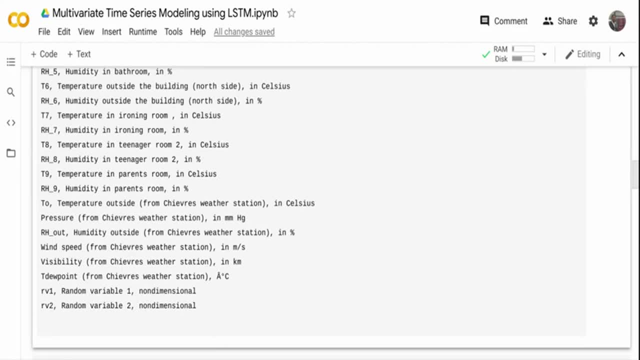 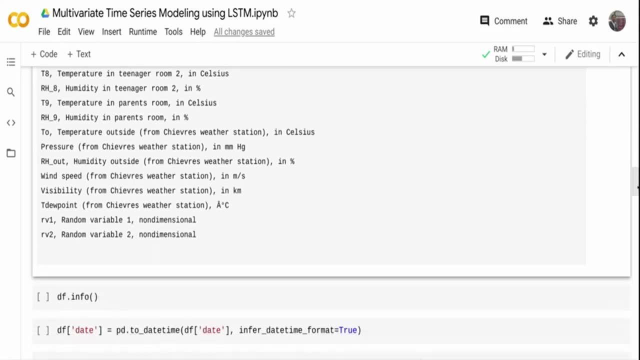 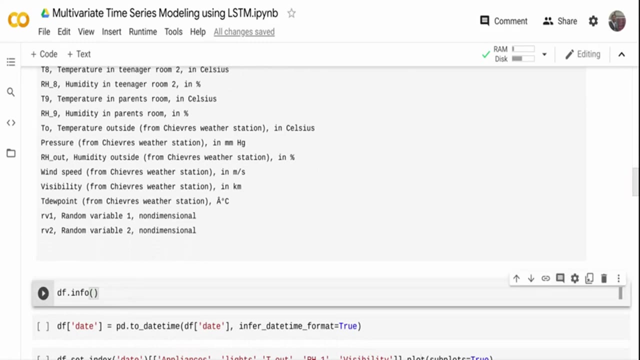 So all this? So inside the house information, temperature, outside the weather house weather information is all captured. So there are 20 variables. But what I'm going to do is I'm just going to use subset of the variable for our purpose, just to demo the multivariate time series. 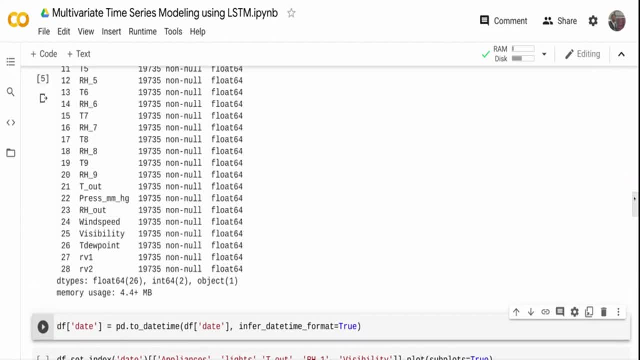 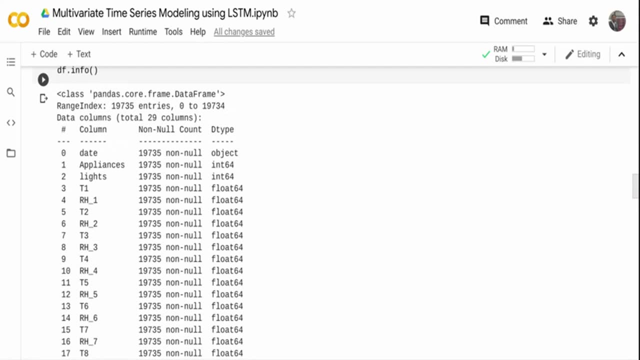 But let's see, like, what is the data type of all these columns? Most of these columns are in float. That's what we want. The date is an object, But in order for us to visualize and make some time series, slicing and dicing- 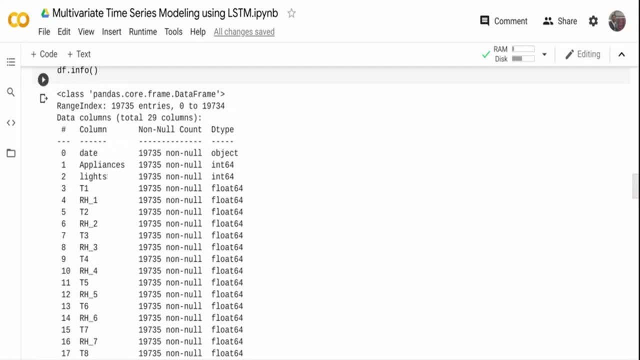 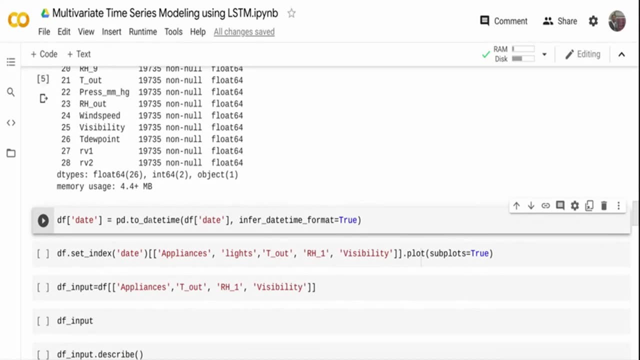 We want date to be in the date time format, right, And the appliances and light is in the integer format, that is, appliances going to be our target column that we are going to use. So what? first thing I'm doing is I'm converting the date column into date time. 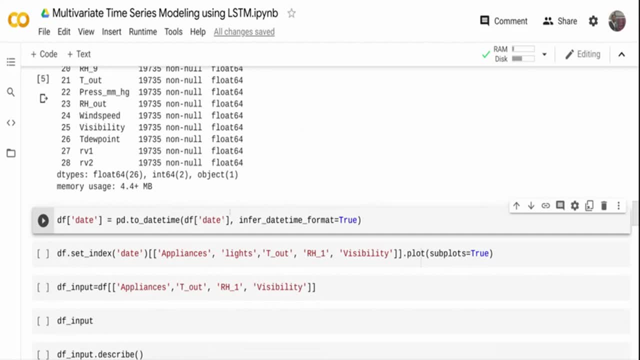 So basically the date column, if you saw on the top, was object. So I am reading it, I'm doing a pandas dot to date time and I'm telling: infer the date format. If you know the date format, if you can also give it, but also you can allow pandas to automatically infer the date format. 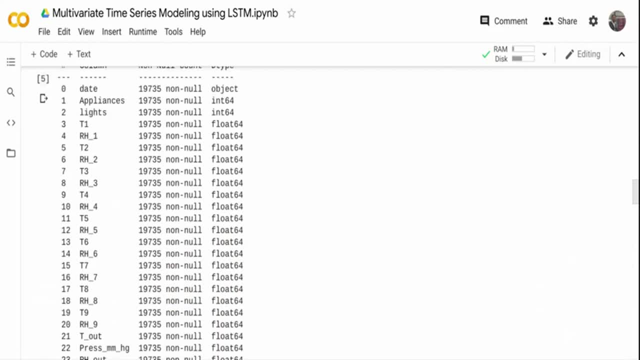 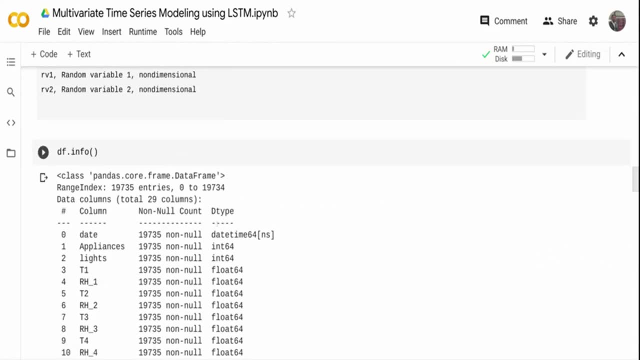 So once I have it, if I go back And basically run this again, you can see the date time is now an object, not. if you see the date times, they're not not an object anymore. It's like a date time data type right now. 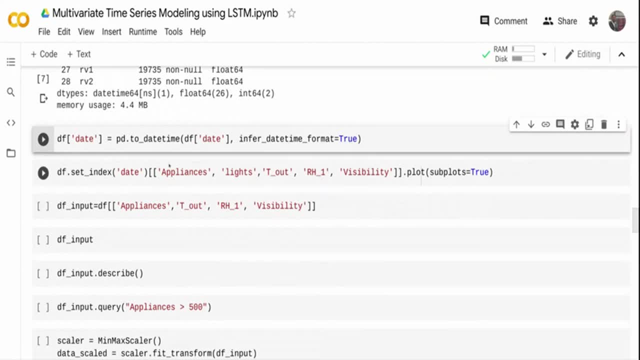 What I'm going to do is I'm going to quickly generate lots of specific columns. I'm not going to use all the columns, So I am setting the date as index and then picking the picking the appliance column: lights, column output, temperature, humidity, And then the 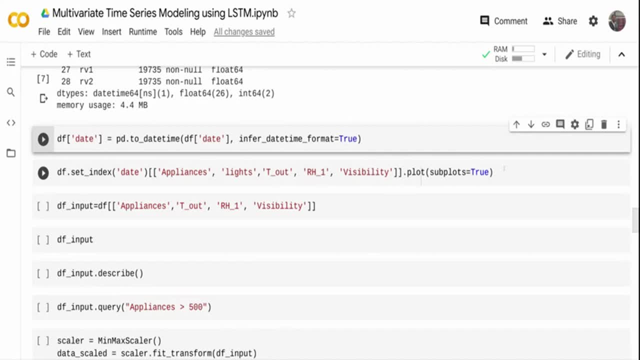 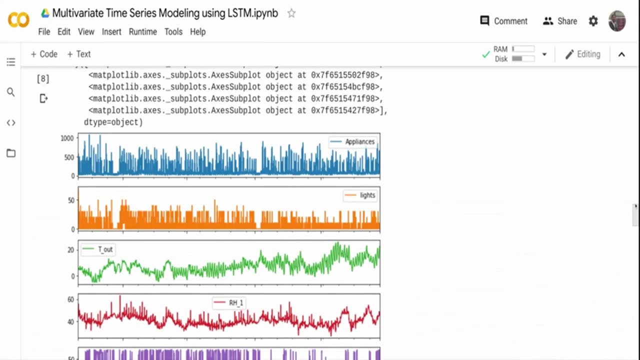 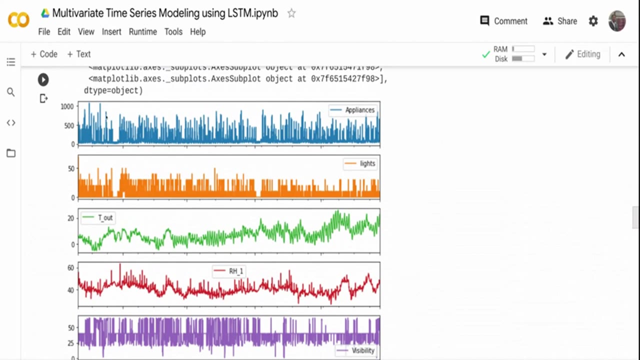 Visibility. So these are the columns I am picking and creating plot of each and every variable. So if you see here you will get like multiple plots And so it looks like. so those are the appliance usages. You can see some spike on the beginning of the year and then it's kind of like 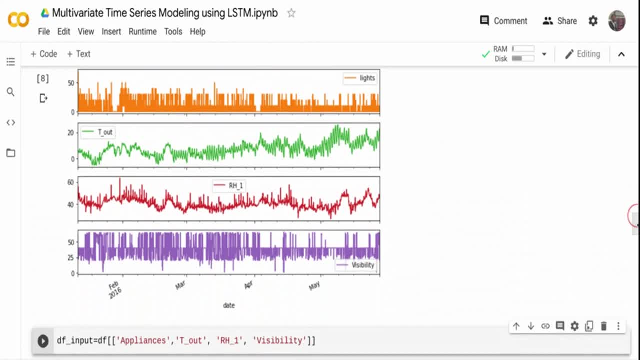 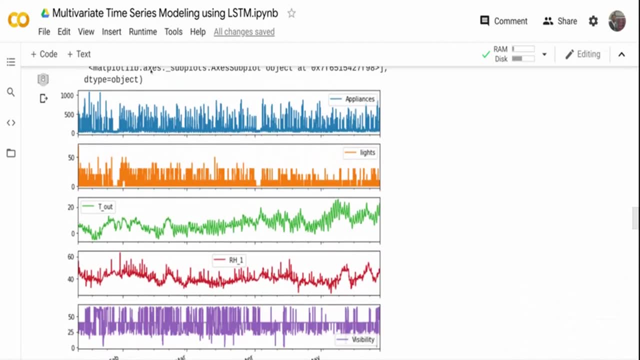 kind of a stable, but there are spikes intermediate right now. If you see, the data is from February 2016 to May 2016.. So you can assume, like the initial month, It's going to be more like winter or it's not going to be hot as the further month. 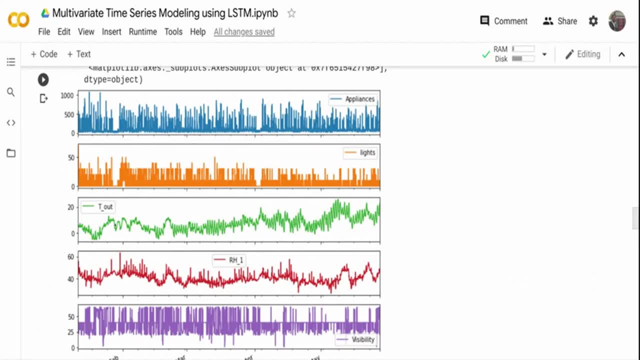 So during winter the usage is higher and you can see that even the temperature out, the temperature is pretty low during the initial month And you can see a behavior that the appliance usage spikes up, And similarly on the light usage as well. The light usage are higher during the winter month because it's going to be darker earlier. 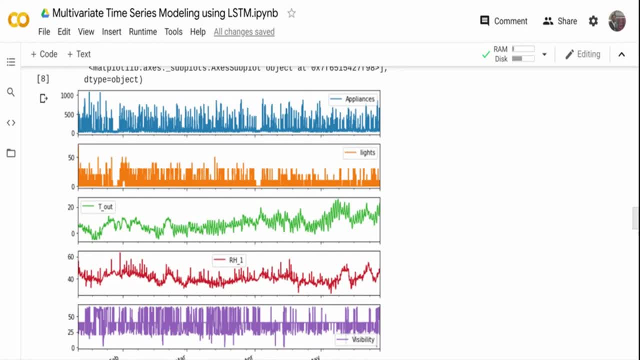 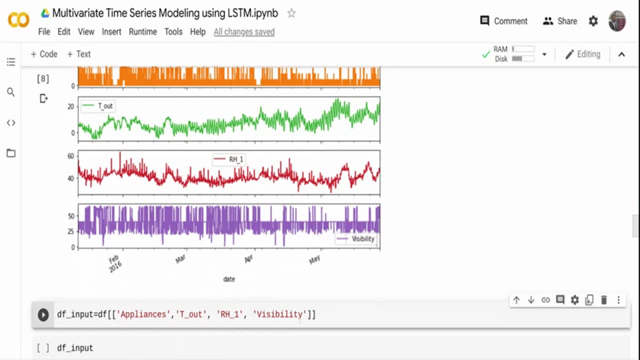 And during the summer it's less Right. So, basically, that is the pattern And similarly you can see, like visibility and humidity, how it correlates. So now what I'm going to do is I'm going to create another data frame. 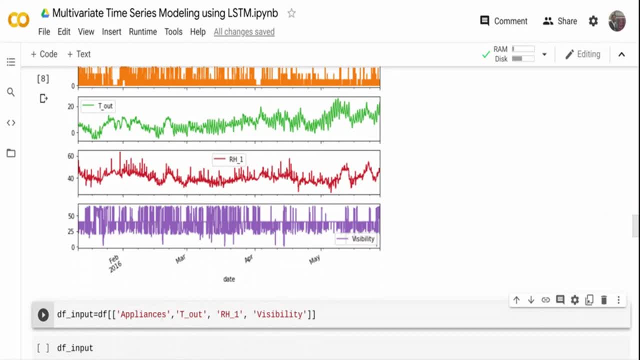 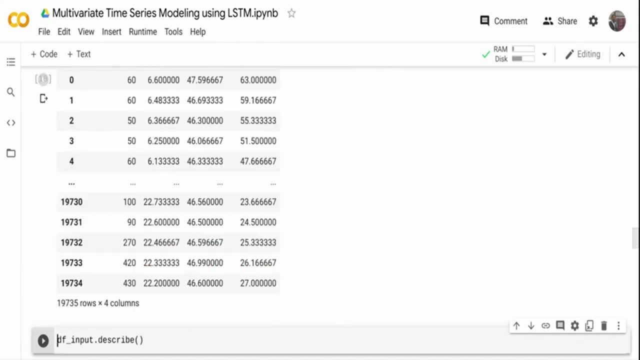 I'm going to use the output, temperature, visibility and the humidity and the appliance as my new data frame. I just created with a subset of column which I'm going to use for my model. So this D of input will have this four columns right. 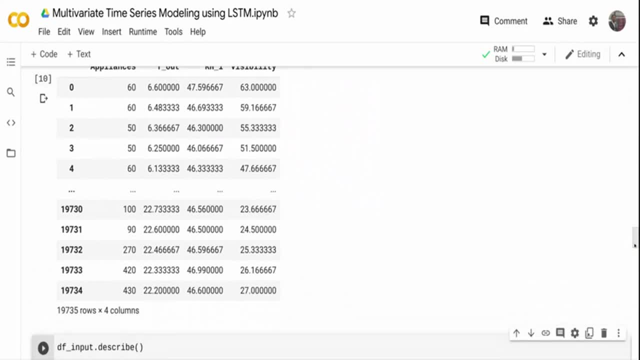 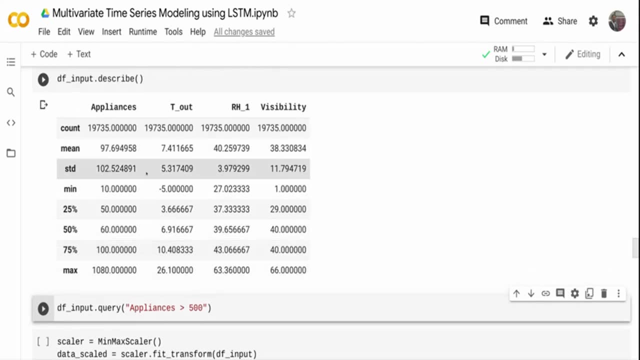 I'm going to use this. four columns are going to be my input in the multivariate time series model. Let me quickly describe the column And just to see like how the distribution of data looks like Now, if you see in the appliance, the 50 percent, the median is around like 60.. 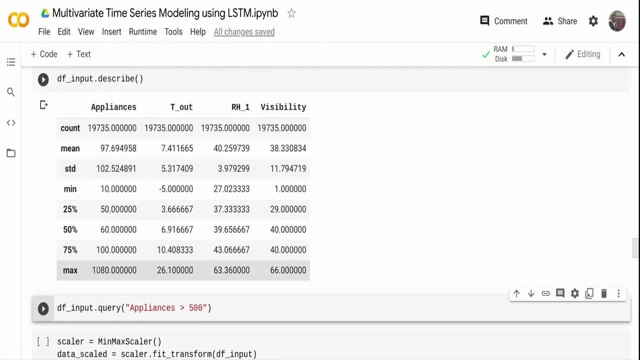 The mean is around 97, but the maximum is at 1080.. Right, So there are extreme values And similarly, the temperature is basically the mean is around seven and there are some max temperature. So, yes, the data is kind of having some some outliers. 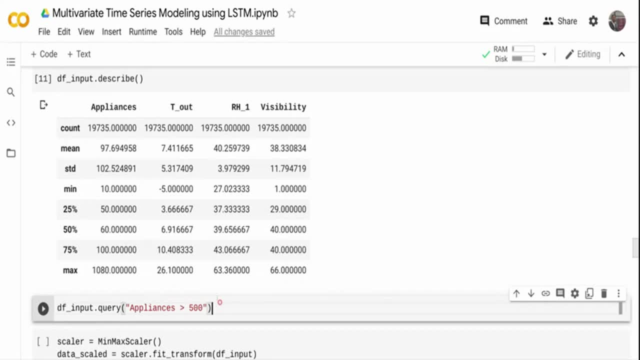 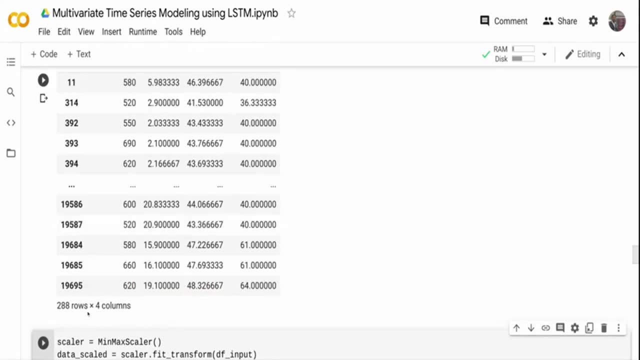 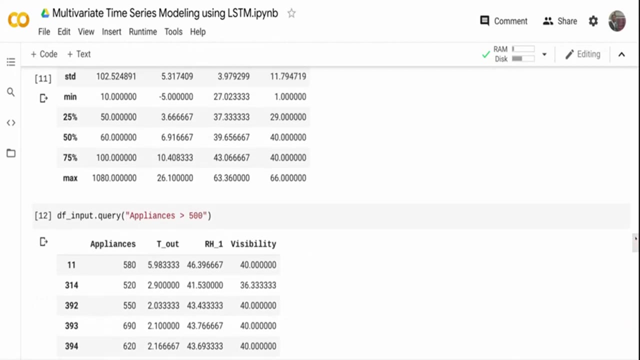 So let's quickly see. Let's take just like some greater than 500 appliance usage and see like how much outliers we have. So we can see around 288 outliers are there. I'm just taking four out of 500. But you can take 100 also, because 100 is the maximum 75 percent value on the top. 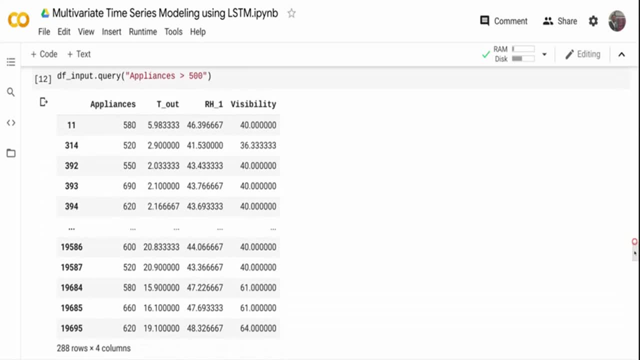 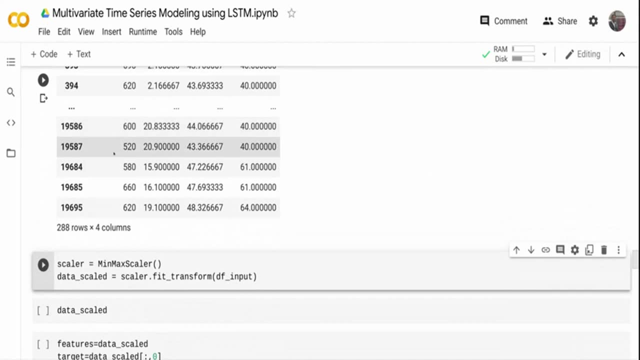 So you can take 100 also, But there are 288 columns. So in order for me to account the outlier, what I'm going to do is when I am scaling it. I don't want to use the standard scalar, because the standard scalar will not account to outlier. 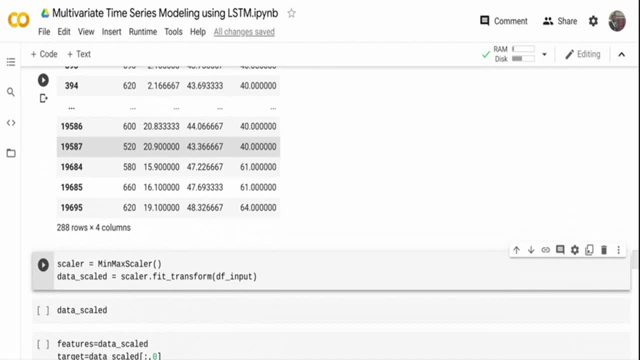 I shift the mean and standard deviation, So I'm using a min max scalar here. The reason I am scaling the data is before feeding into a neural network model, I want the gradients to converge faster, So that's why I'm scaling, so that it has. 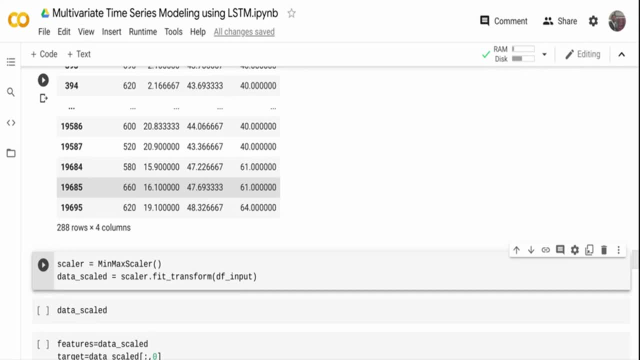 a standard mean and standard deviation for the gradients to converge faster. If you don't scale it, it may take a lot of time to converge. You can try with that also, But it's a standard best practice to scale the data And I'm going to use a min max scalar over here. 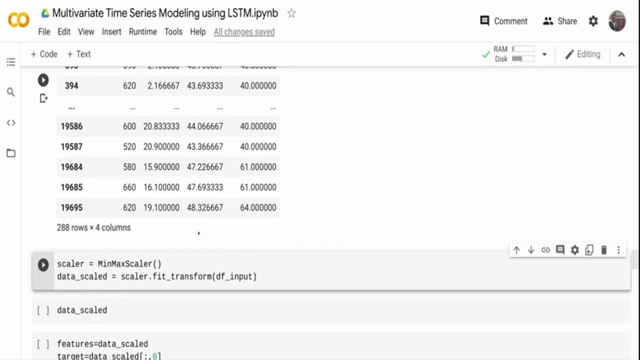 So I'm setting the min max scalar and passing this input data frame. I'm calling the scalar dot fit transform, I am passing the input data frame and I'm getting the scale data. So what the scale data is going to do is it's going to basically scale the data so that it's between like zero and one. 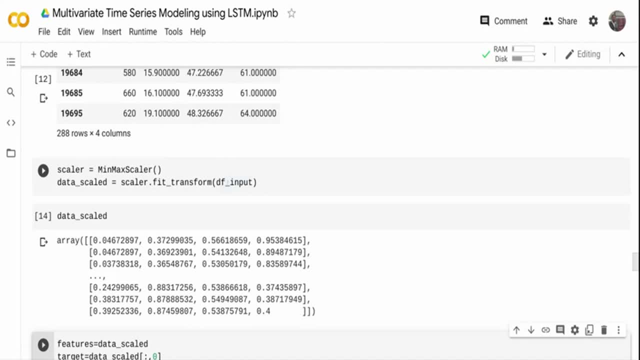 Now what you can do is, when you are having multiple data frame, you can just scale the data for the training data frame and then you can use the scale value for your test data frame, Assuming that the distribution does not vary much. In this case, I just use a single scalar. 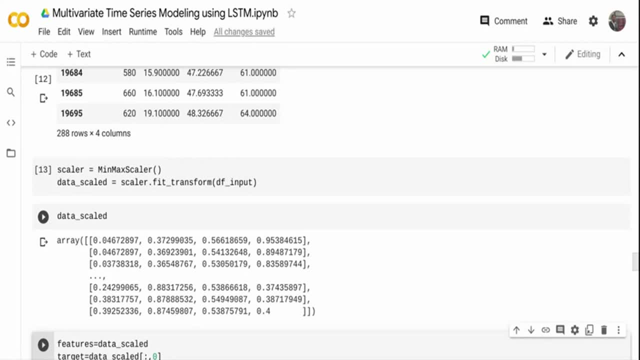 But when you are developing in real time, depending on your data distribution, you may want to take a call. whether you want to, you want to kind of scale it based on the trained value or you want to do like based on the test value. the test is completely different. 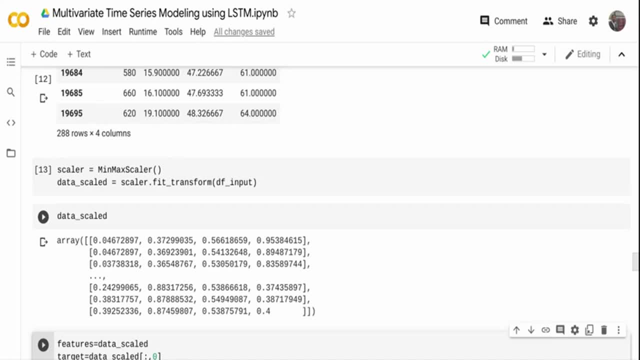 But the best practice is you use the training data frame, You define your scalar on that and use the parameters from the training data frame into your test, And then you can also use the other validation data frames. But in this case that's just done for every data frame. 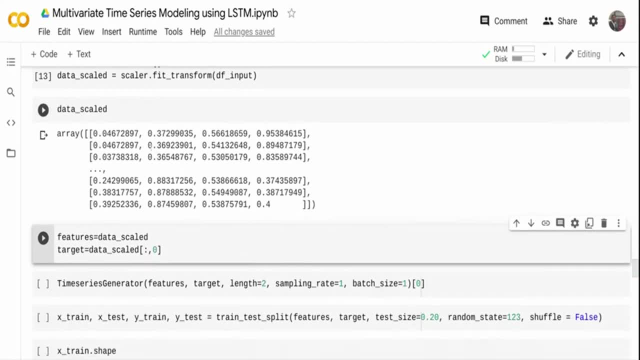 OK, now what I'm doing is from this data, I have defined basically the first four columns as my features. So I am passing all these four columns, even the appliance value. The appliance is going to be my input as well as my target. 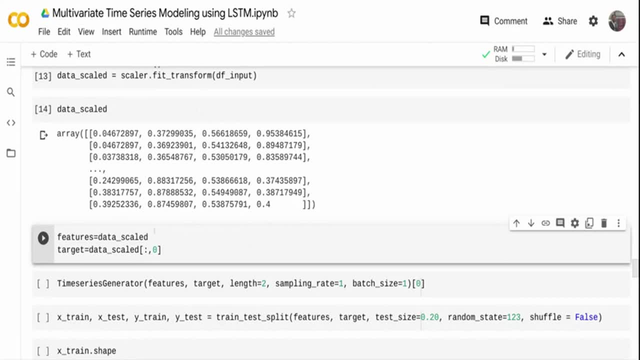 And then the temperature, the humidity and the visibility. I am giving that into the features column and the target column. I'm only taking the zero. That is the appliance. So basically, once I run this, what is going to happen? All these four columns are going to be my input. 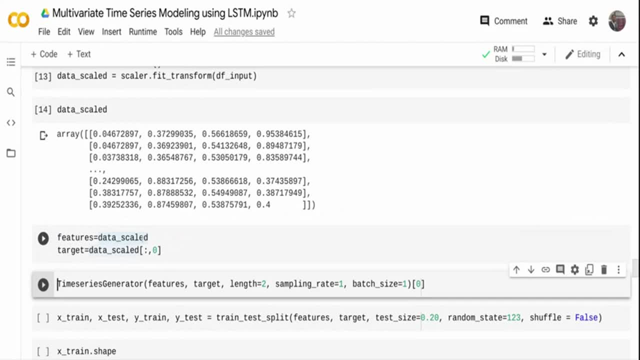 These are going to be my multivariate data to the input of the LSTM model And the target column is going to have only the only the appliance usage value over here. So basically I'm taking the prior appliance usage and along with the temperature and everything. 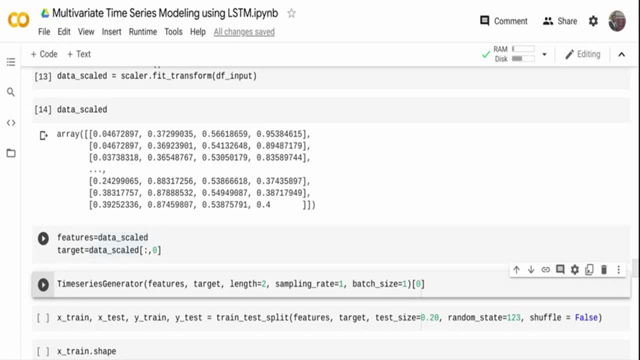 And I am predicting a future value. what it can be, That's what that's what it is. So the appliance is that Passport of input and output, But the output will be a future value of appliance and appliance during the training process will be the current value. 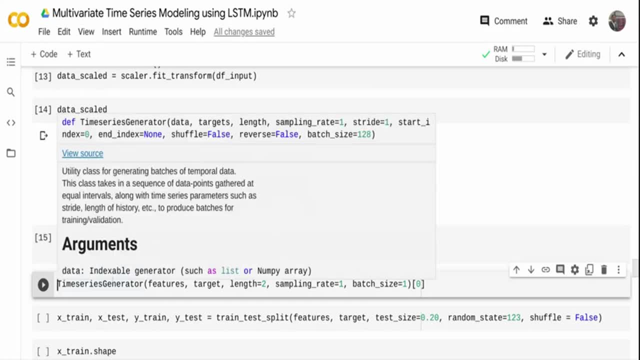 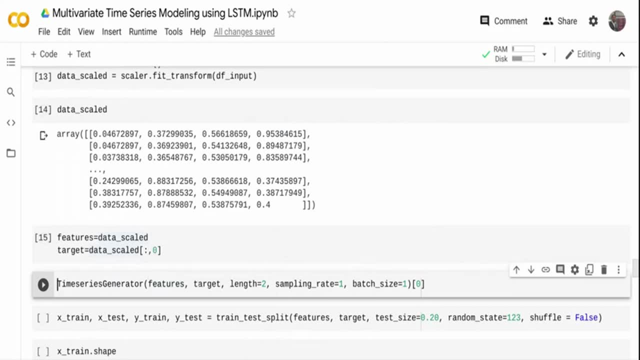 I will explain what I mean by that. So here in the time series generator I'm going to use to prepare the data, I am passing my feature value, which is all the four columns, and target value, which is the appliance column over here. 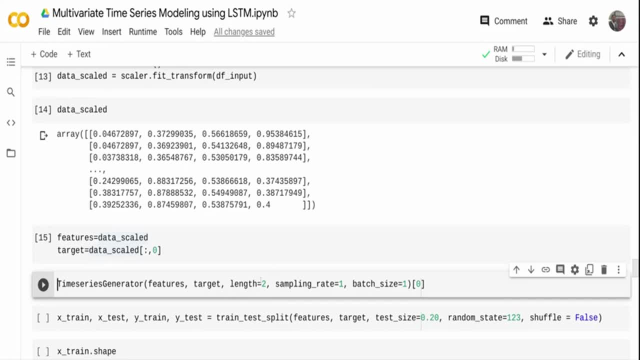 I'm telling my length is equal to two, So my window length. I'm going to take a two time periods of data, So in this case it's 10 minutes data. So basically I'm going to take 20 minutes of data and I am going to predict the next one, right? 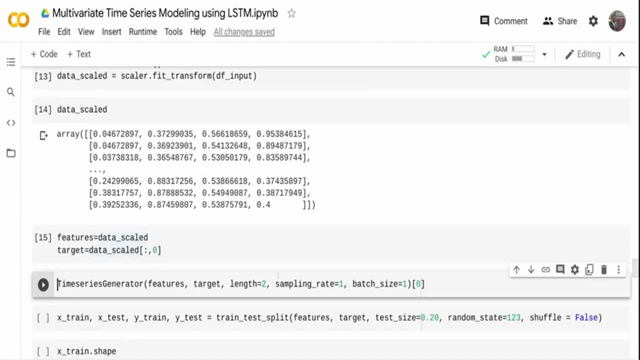 The 30th minute. what will be the value? It is for sample, So I'm just taking the scientist generator. I'm getting the first batch. I've given batch size as one, But in real world you want to give a larger batch size and I'm just printing the output. 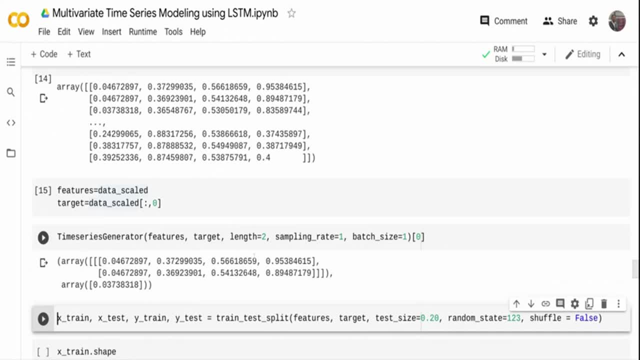 So what we really? what you can see, is it has taken the first training instance. on top There's point four, six and all. It has taken the second training instead. So it has taken two time Periods of data, because length equal to two. 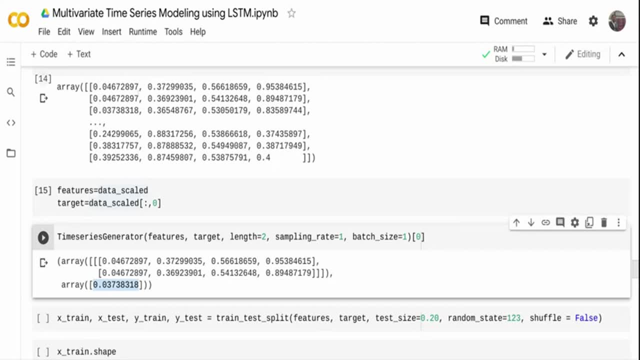 And it's predicting the appliance value of the third. The output is the third. So these two are input and this is the output, Right? So this is how we are going to feed the training data, Right? But? but I'm going to feed for more time steps. 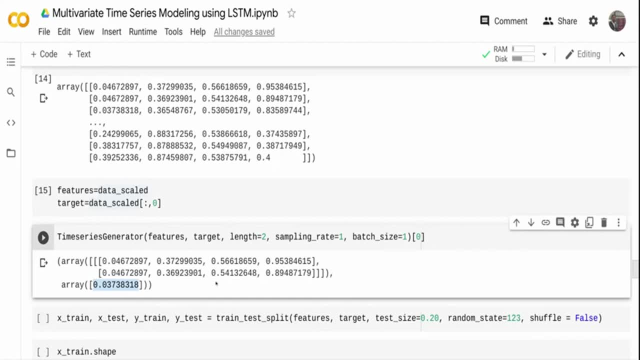 I will come to that, just to show the output. So your input and output will look like: your input will be a list of values of your input, multivariate data, and the output will be your appliance data. So, very first thing, before using the time series generator, 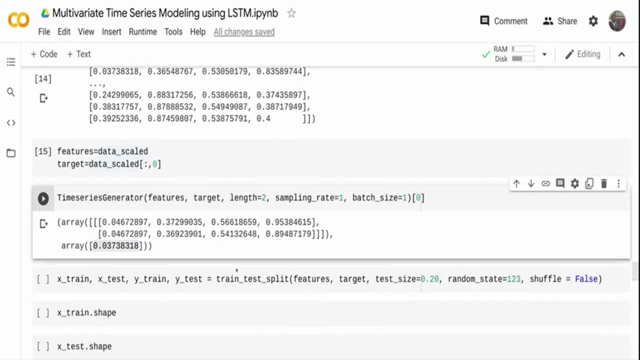 with the real time window. I'm going to split the data here. I'm going to use like: take the futures and target. I'm going to use a train test split and then I'm going to use a test size as 20 percent. 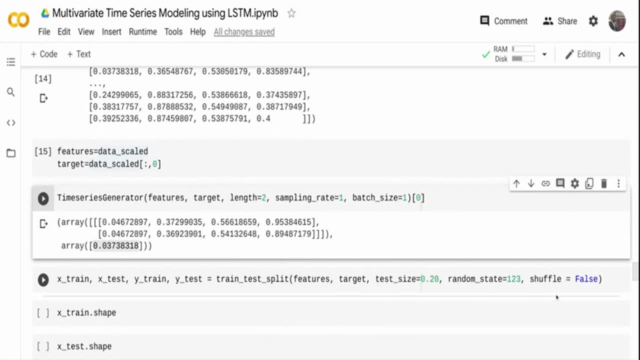 So basically, 80 percent will be training and test size will be 20 percent And I'm telling shuffle equal to false. This is very important because it's a time series data. The order is very important. If you don't give, it will become shuffle equal to true. 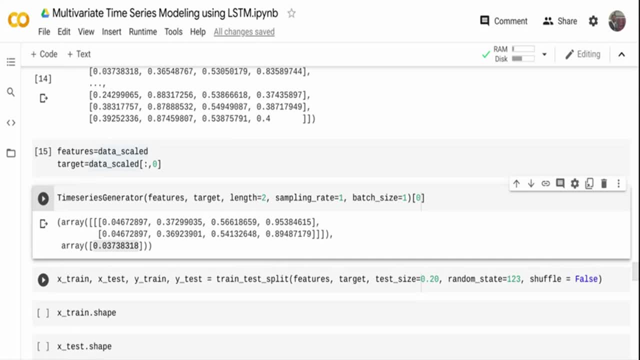 So it will randomly shuffle. You can split the data, So you're losing the order. When you define a LSTM model, you don't pass time at all, You just pass the features. But when you're defining a Facebook profit model, time is an input parameter. 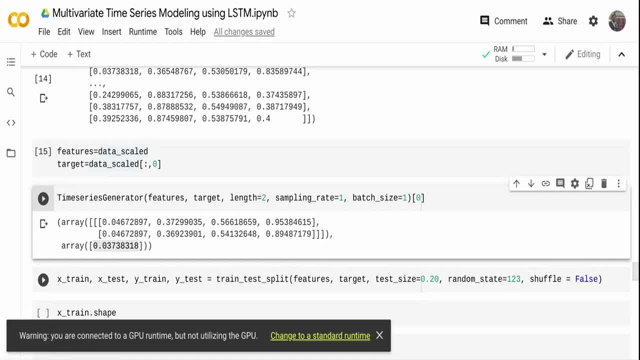 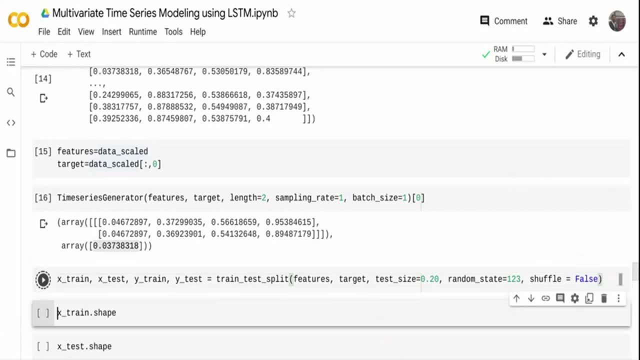 Right, But so you need to make sure that when you are passing the data, the data is in the same order, Right? So what? what I'm going to do is I'm going to split the data, test and train, and you can see my train shape and shape. 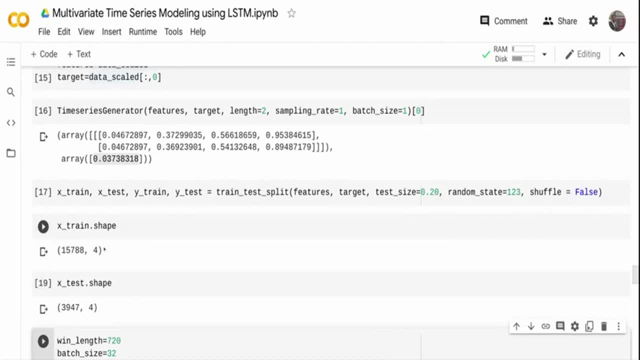 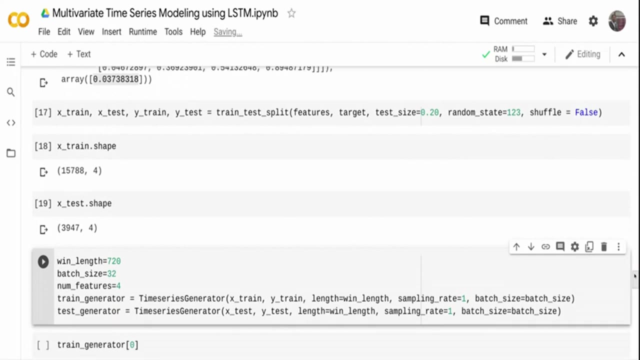 or your trainers, around fifteen thousand seventy eight instances. There are four features. And then test around thirty three thousand nine hundred forty seven instances and four features. Right Now I will define my time series generated actual time series generator that I am going to feed into the model. 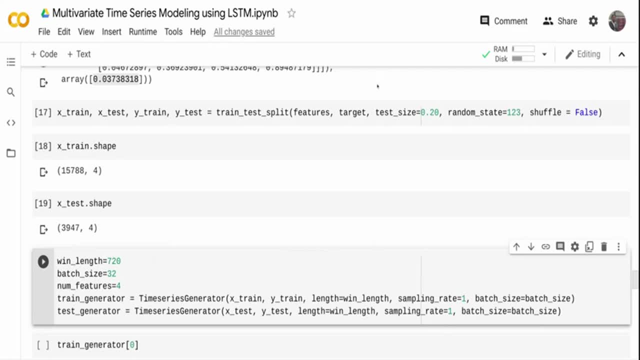 So what I'm doing I'm defining the window length. in the previous one I gave window length to two. That is just for sample. I mean you're defining the window in the seven twenty. So what the seven twenty means is: I have data every ten minutes. 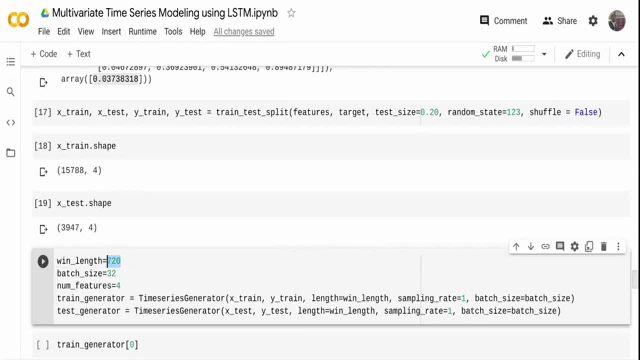 So for ten or so. for one hour I have six data points. Twenty four hours I have twenty four into six data points. So on a day with ten to ten minutes interval, I have one forty four data points. I am taking five days of data. 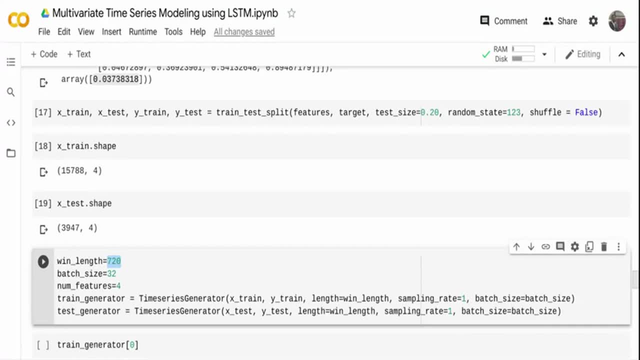 So that's why it's seven twenty one forty four into five. So each day I have one forty four training instance. I am taking five days of data and using this five days of data, I am going to find the next observation And that's why I've given window length of seven twenty. 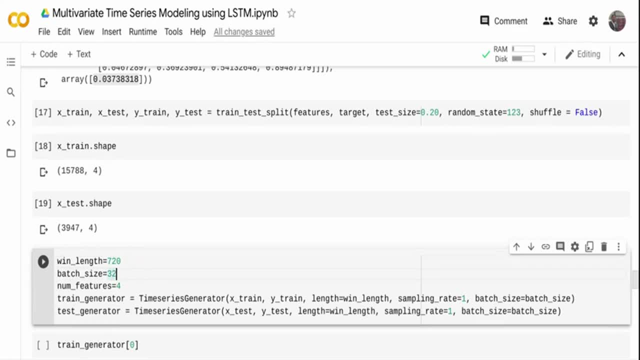 I have given batch sizes thirty four. I don't want to train one, I want to train one record by one record, because I need my training to be faster. I am defining a batch size of thirty two so that in each training instance I am. 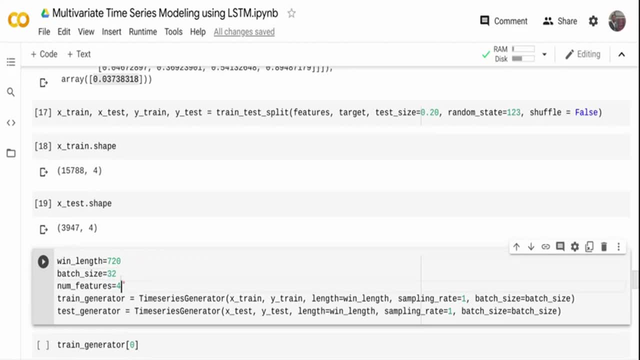 passing thirty two batch size of data and then the number of features is four. That's our input feature size. That is four And I'm creating a train generator and test generator. in the train generator I am passing the X of train and Y of train, which is nothing but the 80 percent. 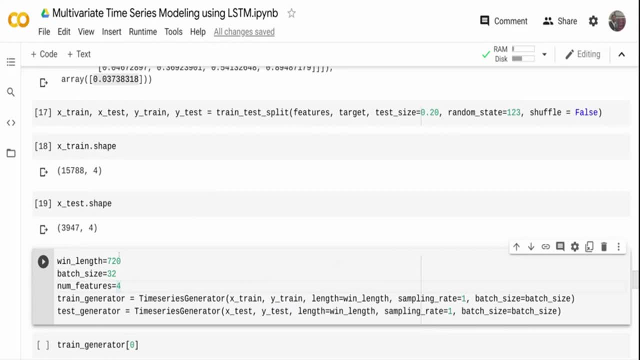 of the data I am telling- my length is seven twenty over here- which is, take five days of data and predict the next instance. The sampling rate is one and the batch size is thirty two And similarly I'm defining the test generator based on X test and Y test of Y test data frame. 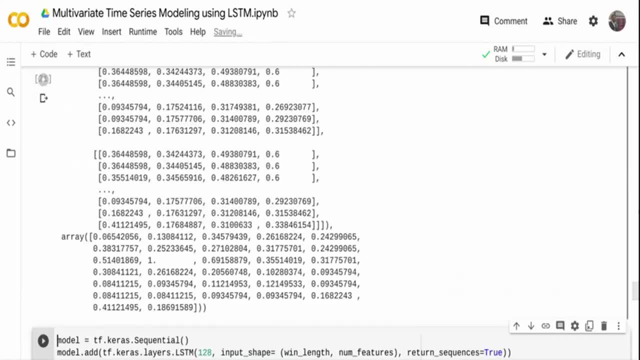 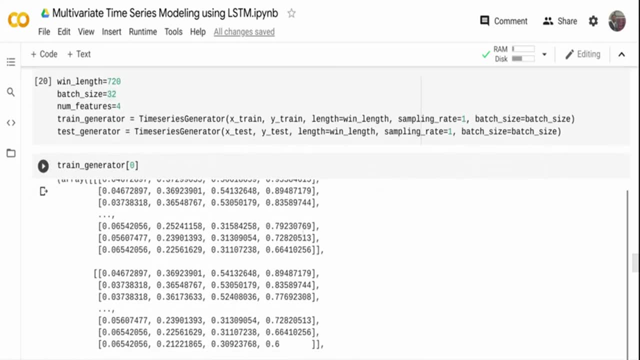 So quickly. then we put the train generator and you can see. basically it will contain thirty two, because the batch size is thirty two. It will contain thirty two observations, each of length, seven twenty, each of each having seven, twenty observations and each observation having four features. 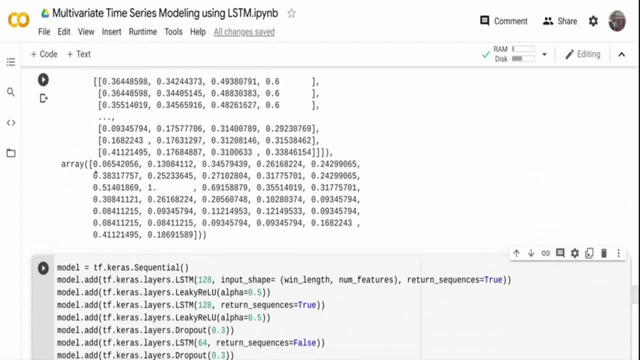 And then, finally, you can see that will be the target column. It will be thirty two target columns because there are, it's a batch size of thirty two, Right? So that's how it looks like. Now we will go and define our, define our model architecture. 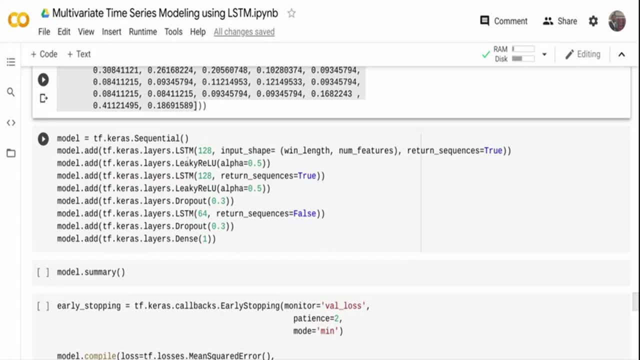 So what I'm going to do is I'm going to define an LSTM model. I have multiple layers here. Here what I'm doing is I'm creating a sequential model instance and then I'm telling my LSTM layer: basically, number of units is one twenty eight. 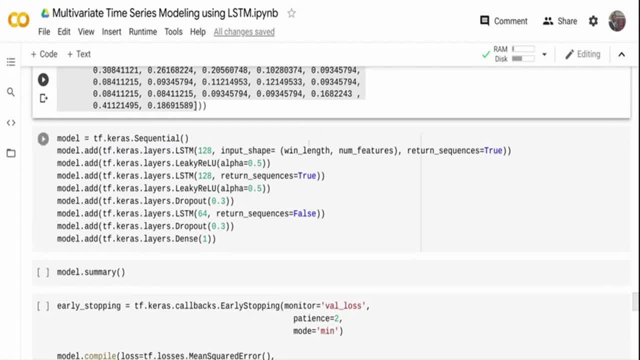 My input shape is my windows length. Window length is seven twenty on the top and comma four. So basically I have seven twenty instance with four features. That's my input shape. And then I'm telling written sequence equal to false for written sequence equal. 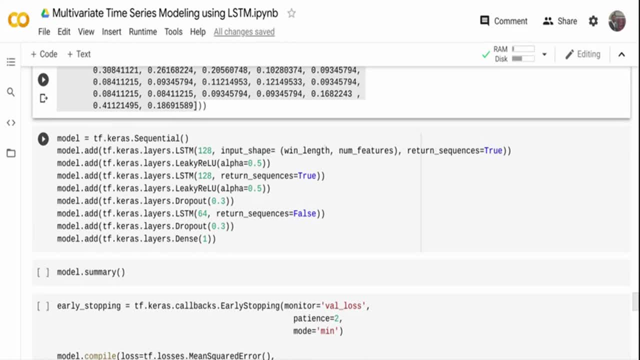 to true, and why you give true is basically now you need. you need a hidden state for each of my input data. If I give it false, it will only return one hidden state for all the input sequences, But here it's a time series data. 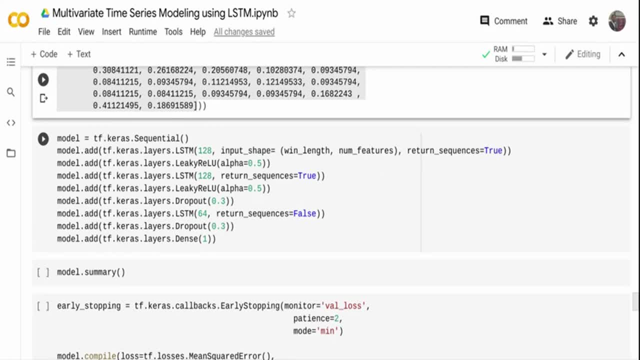 I want to take each and every observation into account, So I need to have hidden state for each and every observation, and that's what the written sequence does. Right, I'm using a leaky reload activation function And then, similarly, I have one more layer with another one twenty eight. 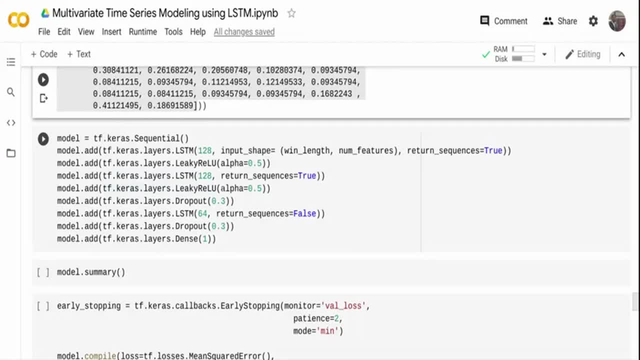 one twenty eight LSTM layer, And again I have a drop out just to make sure it does not overfit. And then again I have an LSTM layer with sixty four. And here I am telling. written sequence is false, So in this case I will return only one. 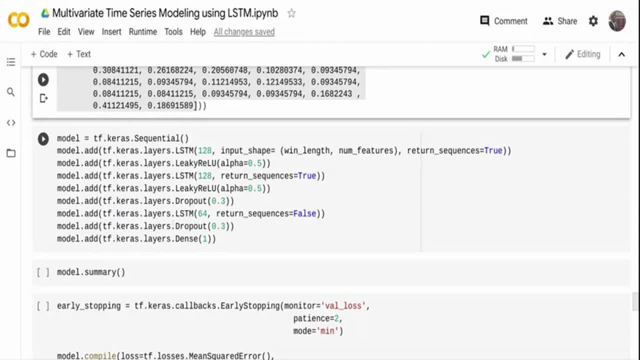 It will only one hidden state. I can still return true and I can have a dense layer. I can flatten it, I can have a dense layer, But here I'm just creating false and I am creating a final layer of one which will basically give me the final. 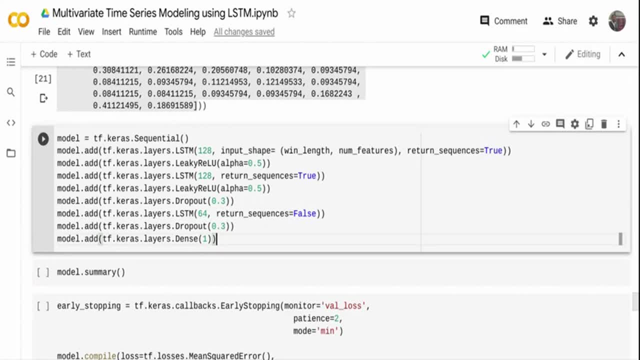 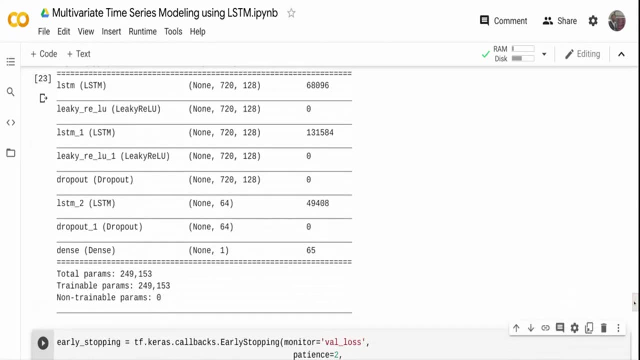 prediction of what is the appliance usage in the next hour, based on the input data. So this is my model architecture. Let me quickly run my model summary and basically You can, you can see over here how this particular model looks like. OK, this model has around two for two, fifty thousand parameters. 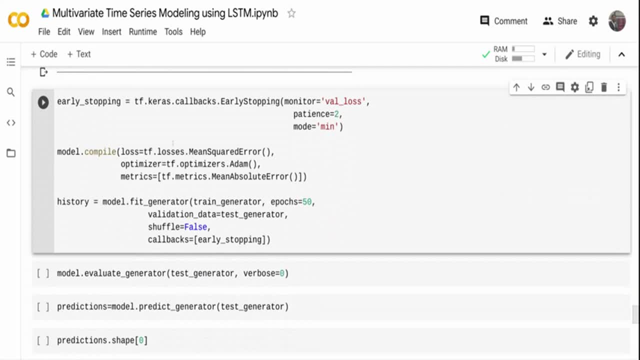 Right, Then I am defining my model. So what I'm telling? I'm telling early stopping. I don't want to run forever, So I am giving like fifty I to a box here, But I'm also giving early stopping. that is telling if the validation loss. 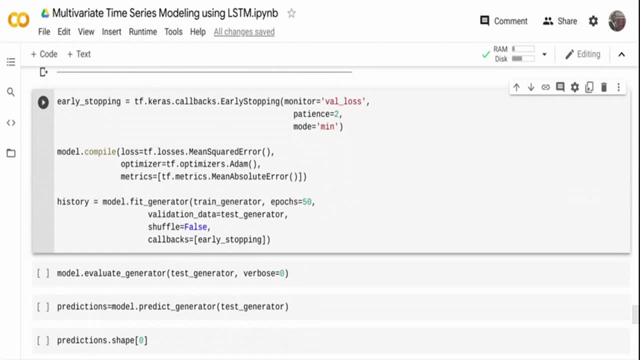 is not improving. at least two iterations, then basically stop the training. Right, That's the early stopping Keras callback. I am compiling the model using a mean square error And my optimizer is Adam and I am giving the metrics to monitor this mean absolute error. 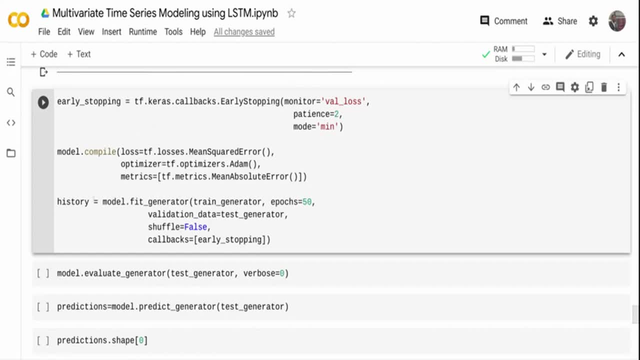 Right, That's what I have given over here, And I am calling model to fit generator. You can also give model to fit with this, But I'm giving model to fit generator. I'm passing the training data frame and then I'm telling my box is 50,. 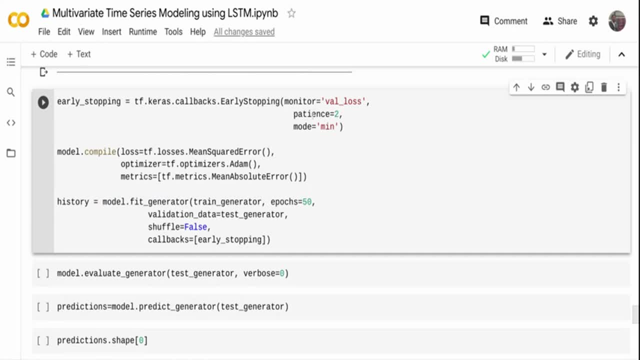 but it will not run for 50 bucks if the model sees it's not improving to stop based on the early stopping. So that's the early stopping. Keras callback. I'm telling shuffle equal to false. We must not shuffle the data by default. 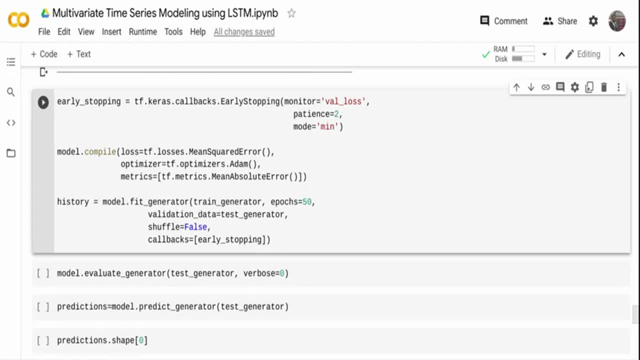 Right. So because the time series data- the order is pretty important- and telling shuffle false. And then I'm telling my validation data as test generator. It's typically good to have one more slice of data for testing the data, But here I'm just using the validation data for both the purpose. 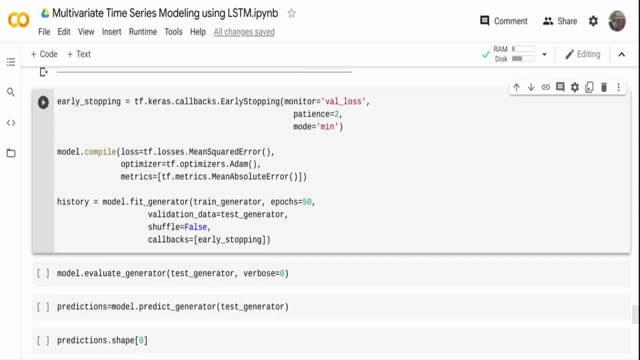 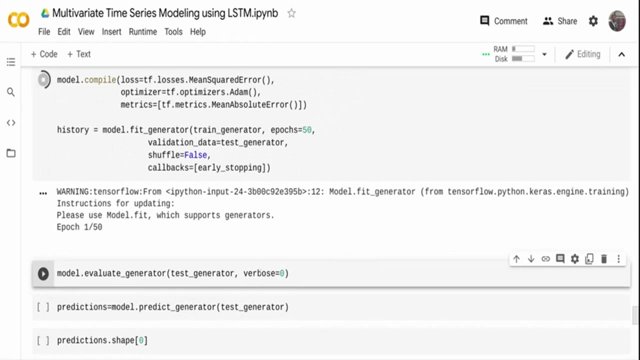 It is good for this video, but in real world, you may want to have trained data, validation data and test data separately. So this is the model architecture. Let me quickly run this. It's going to take some time to train, So what I'm going to do is I'm going to wait for it to complete and then come back. 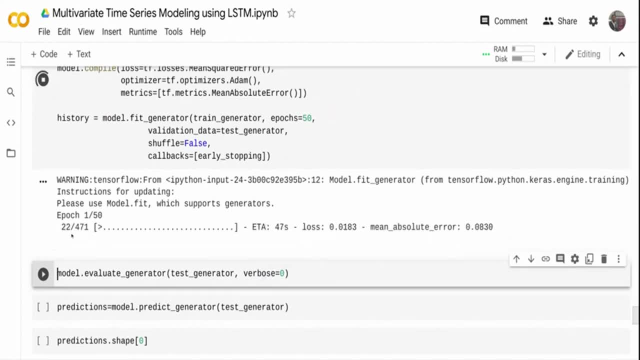 But let's quickly see one epoch so you can see basically it's training and make sure you have GPU on. even without GPU this will work. Only thing is it will take some time. I have set GPU in the collab so you can see basically the loss is decreasing. 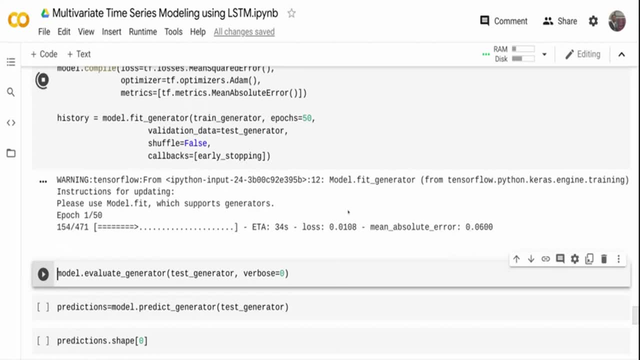 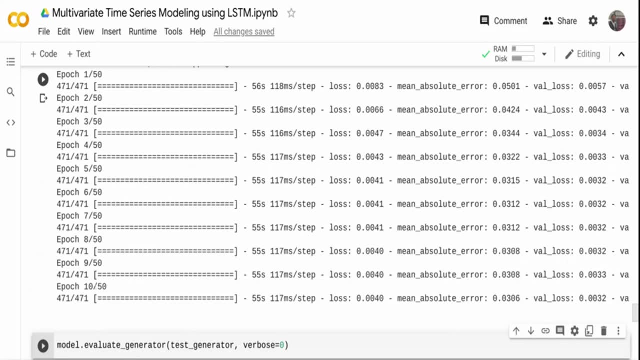 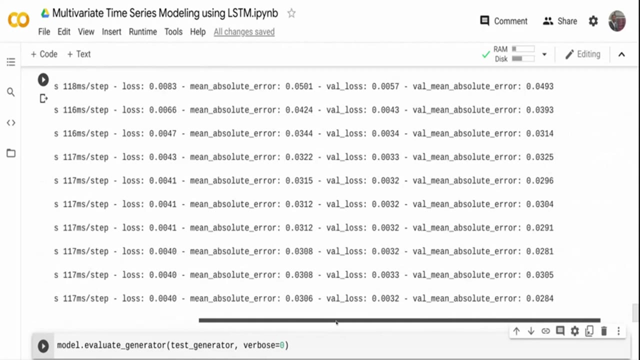 The mean absolute error is there. So I'm going to let the training complete and then I will come back and continue with the video. So model is trained now. It took 10 epochs to train because of early stopping it stopped And basically you can see over here like the mean absolute error validation is. 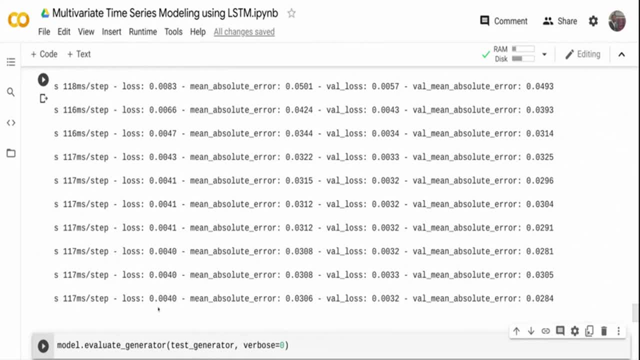 0.284 and the loss is 0.040.. Basically, the training mean absolute error is 0.03.. So this is the model we have got. Let's see how well this model performs with the test data that we created. 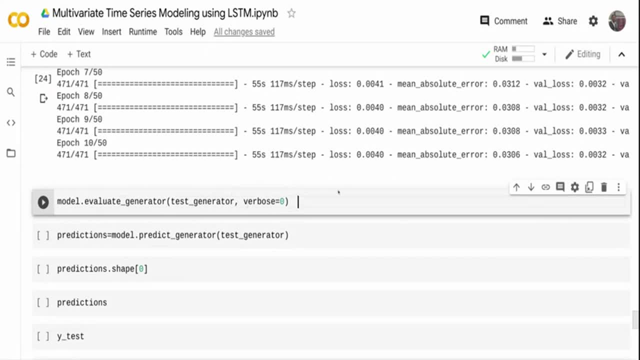 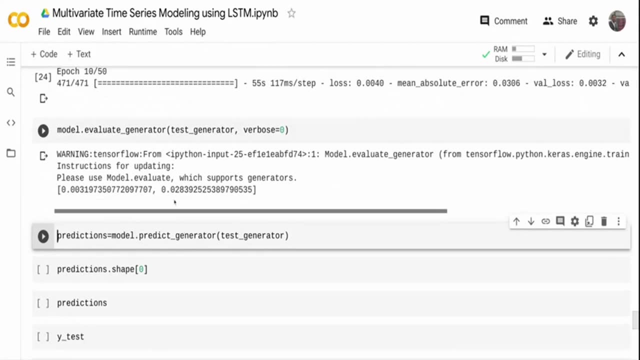 So let's evaluate this particular model with the test data that we have and see, like, how it performs. So basically, you can see the mean absolute error is 0.028.. What I'm going to do is I'm going to go and predict the value and I'm going 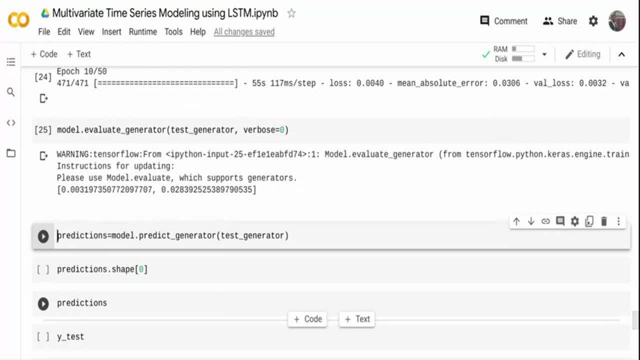 to compare it against the actual value of the model did. Okay, So I'm calling the model dot predict generator and I'm passing the test generator. I'm getting all the predictions Now once I pass this. if you see basically our test data frame at: 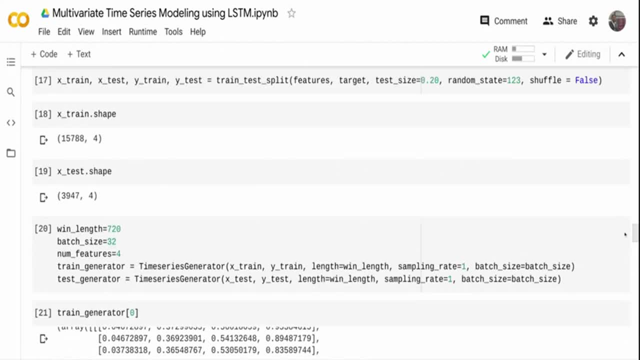 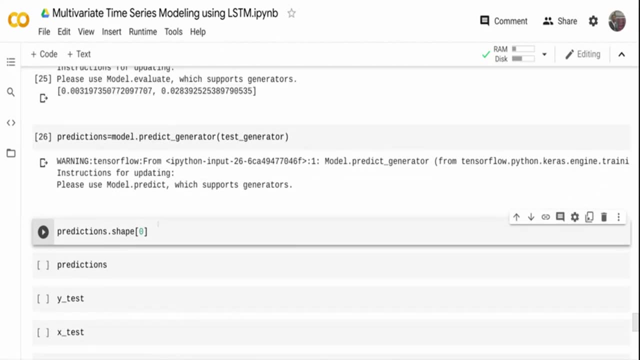 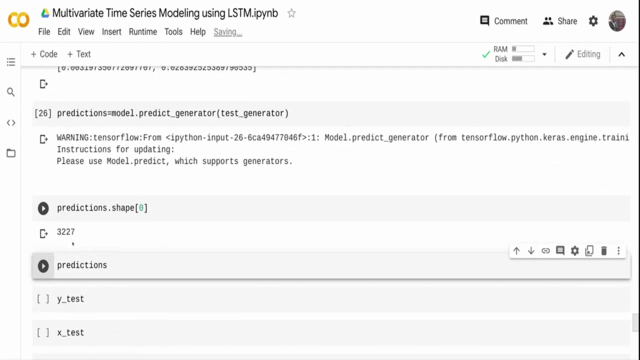 some 3984 records, or something like 3947 records. right, The test generator. So once it's done, let's see the shape now. So it has only 3227 rather not 3947.. The reason is: you can see, there's a difference of 720, and 720 was our time step. 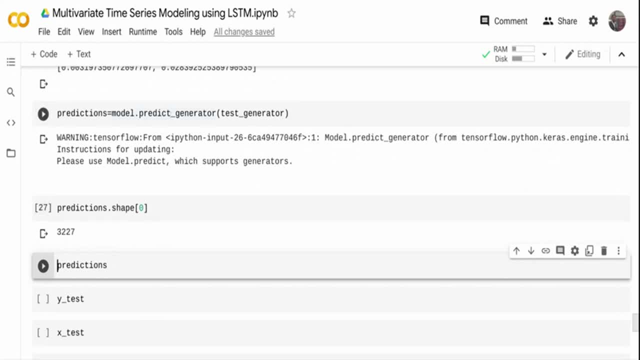 So when you are passing the data to the prediction, it's going to take the first 720 columns to predict, the next, next and after. this is going to keep on sliding next, next, next to all the values, So you will always have numbers less than the windows length. 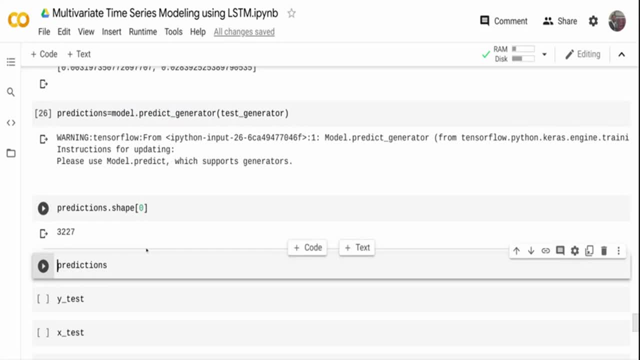 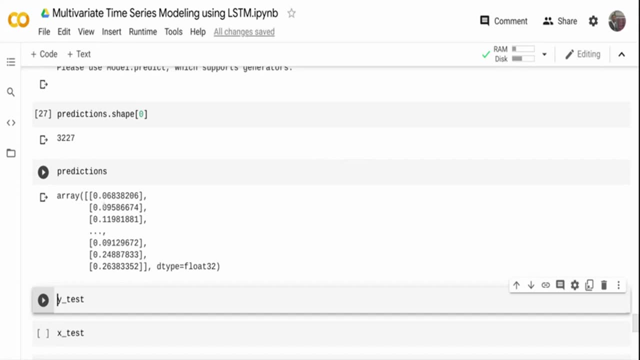 The window length is 720 for us, Right. So let me quickly print the prediction. And if you see this is the prediction, if you actually see this is the appliance output, but if you see our actual data set, the appliance output was like 60,, 70,. 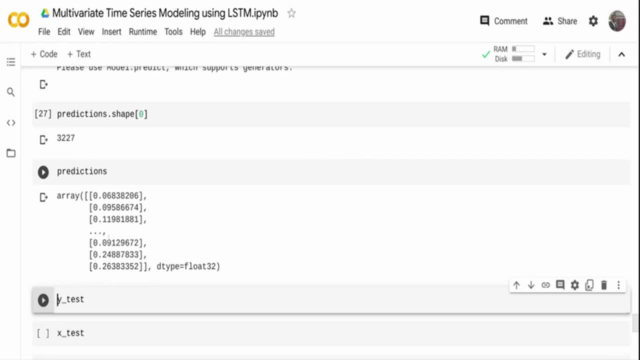 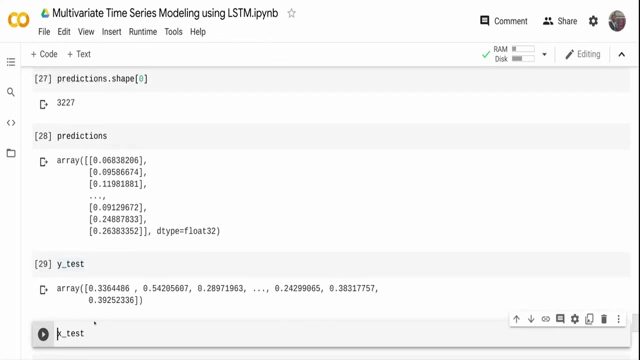 100, a whole number, And this actually scaled prediction. Now we need to do a inverse of the scaling and get back to the original prediction prediction and compare our model of it has performed right. So let me quickly print the y test And if you see the y test, this is what it looks like. 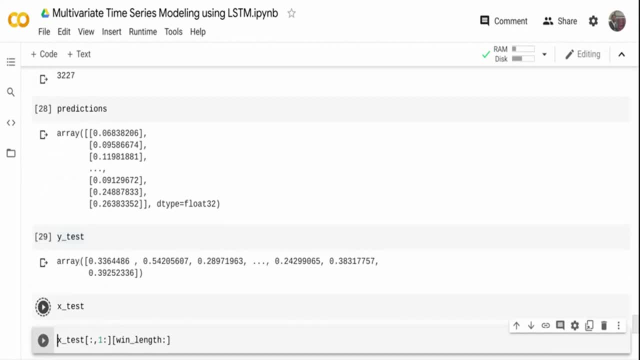 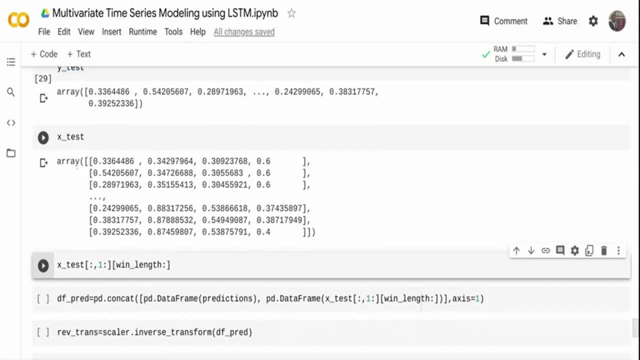 The point three. three, and this is what you can see Right, Basically, y test is also a scaled value. Now, what I'm going to do is I'm going to take from the x text. So these are all the different data that we had, Right? 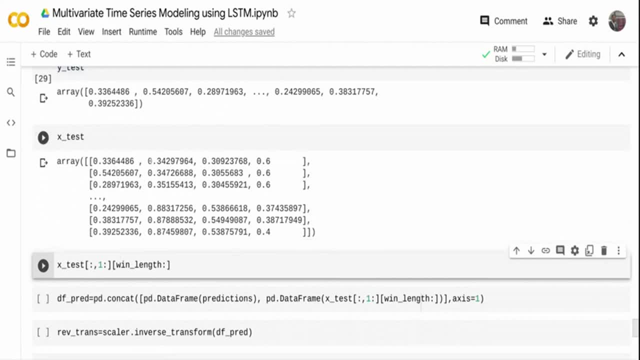 I'm going to take the all the data from first column till the end and from the windows length. So window length is like 720.. So I'm going to ignore the first 720.. The reason is our prediction value does not have the first 720. 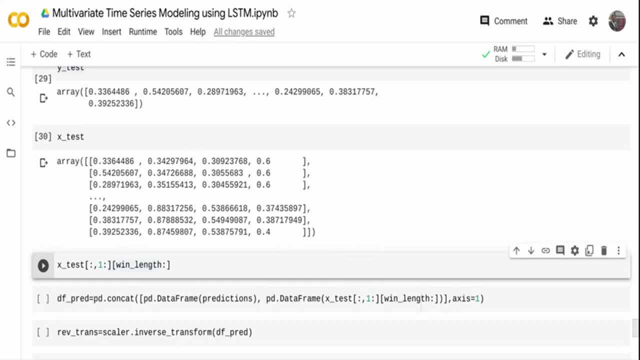 It has only three thousand two forty seven records or something like that. Three thousand two twenty seven against like three thousand nine forty seven records that the actual test data had. So I'm just taking the knowing, the first 720, and taking all the value. 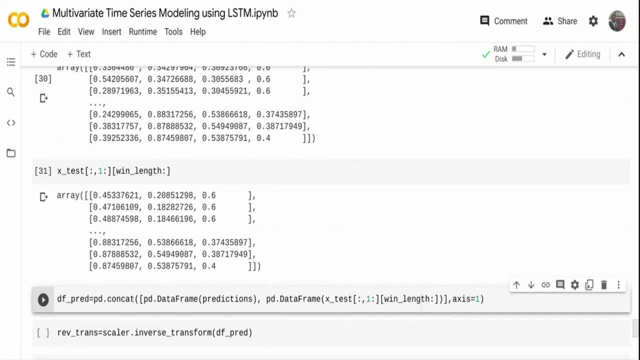 I am going to create like a concatenation of the data frame. I'm going to take all this from the x text and then I'm going to take the predictions from what we got And I'm going to concatenate and build one final Pandas data frame. 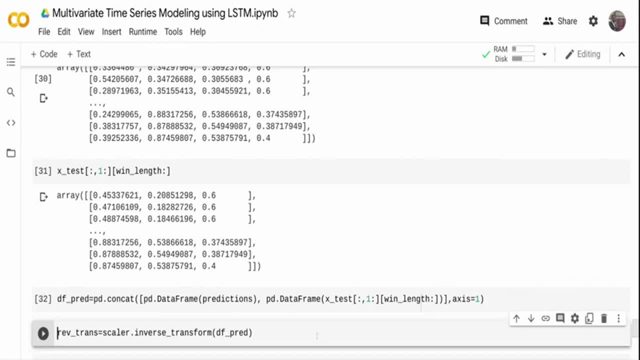 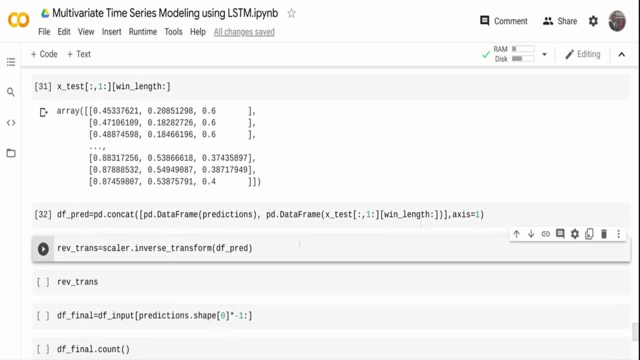 So basically, I here I will have like a data frame which will have the predicted value and which will have all the value. So I'm going to take all the values from from the x text. rather than having the actual label, I have the predicted label. 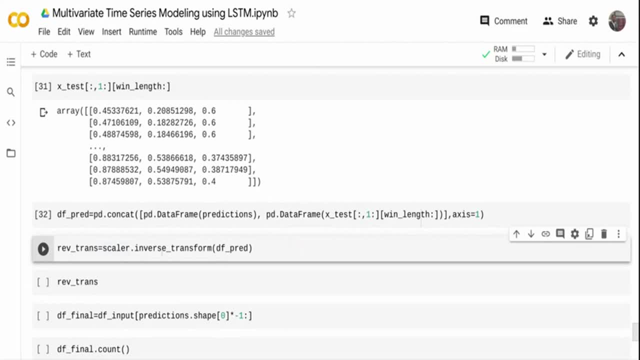 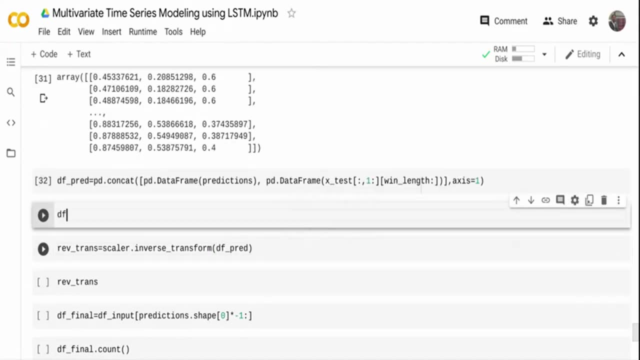 That's the change I have made And I am going to take the scale that I created on the top and I'm going to run a inverse transform and I'm going to pass this predicted value. So if you see, this particular DF Underscored, right DF. 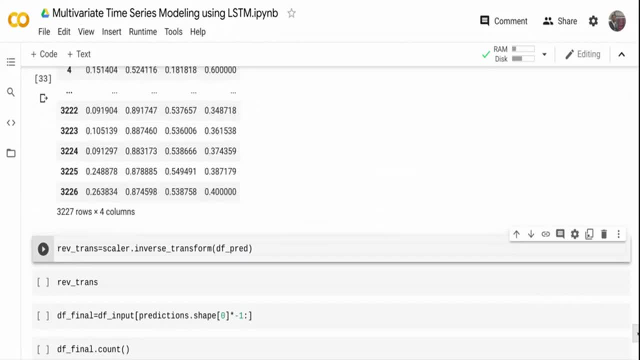 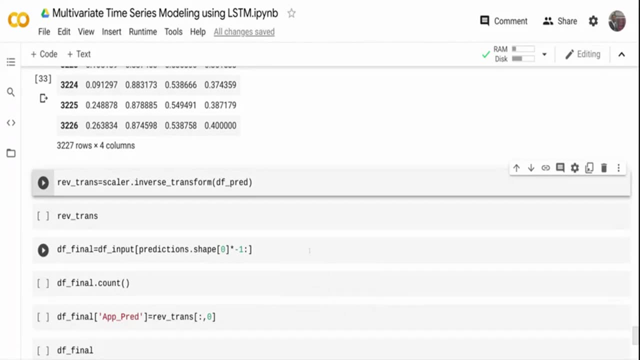 Underscored. right, it will have these four values over here Right now. these are all scaled values. I did a scaling on the top. I use a min max scale. Now I need to do a inverse transform. That's what I'm doing over here. 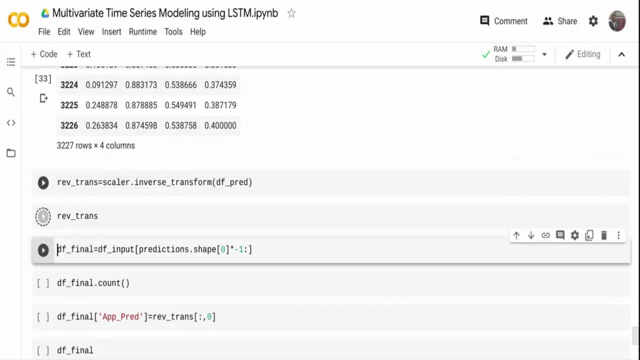 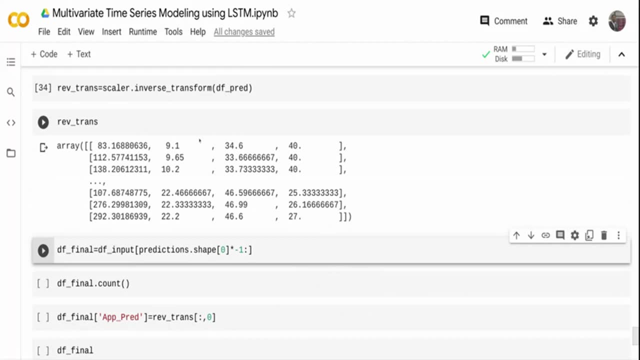 So once I run this inverse transform- and now let me print the reverse transform- you can see the values into the original format, Right So? so now I have this data frame over here, Basically I have all the columns and I have the predicted value right now. 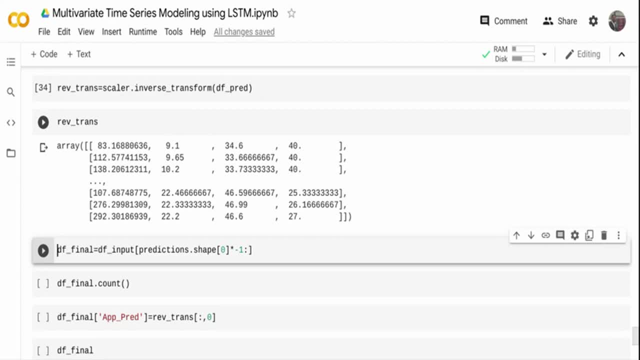 I need to take this predicted value and compare how close it is to the actual value, Right? So what I'm doing in the DF input data frame that we created on the top Is the actual data frame. So the first 80 percent is the training data. 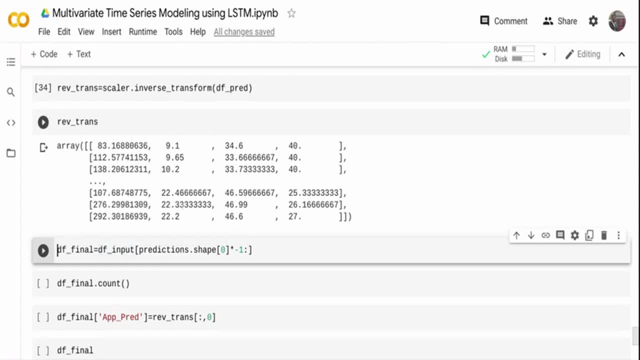 The last 20 percent is what we use for prediction And that is what it is over here. So basically, what I'm doing is I'm taking from the DF Underscore input. I am getting the prediction shape. So the prediction shape is what it is actually: three to four, seven or something. 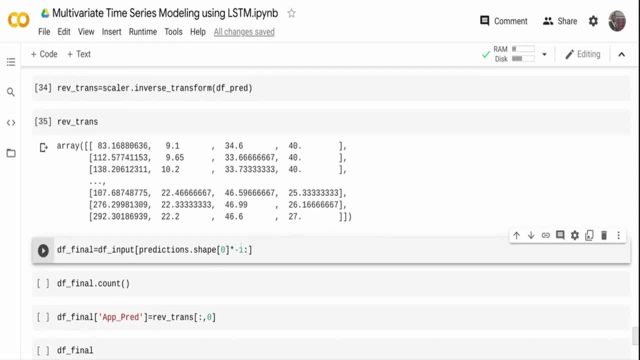 like three to two- seven Right, And I am getting the last three to two- seven rows. This last two three to two- seven rows is basically our prediction frame that we are using And that's what I'm doing over here. 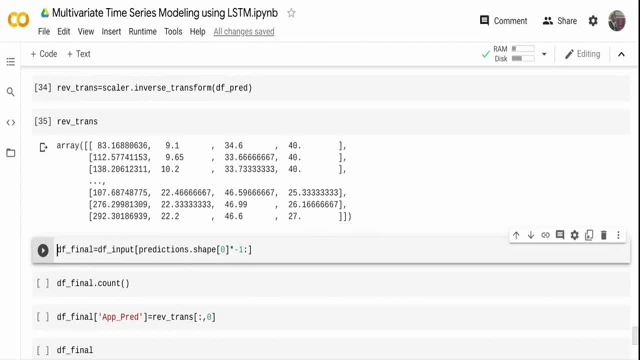 So basically it's going to take the line when I say minus into minus one. Basically it's going to take from the bottom to top. when I don't give minus, It's going to just take top to bottom, whatever size we are given. 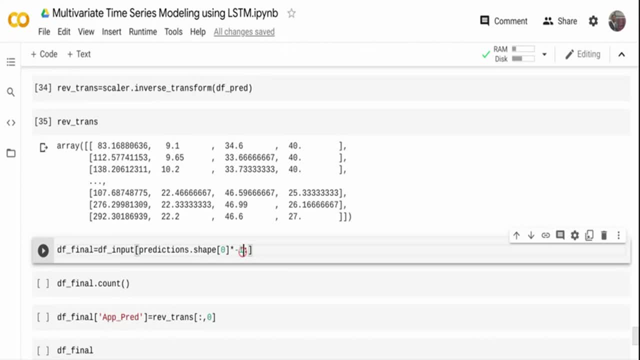 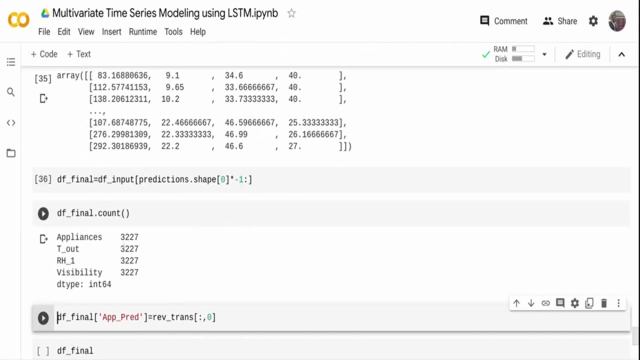 But here I am doing minus one, So it's going to go from bottom Right. So once I have this DF, finally data frame, if I do and kind of count, you can see it as three to two seven, which matches our prediction frame on the top. 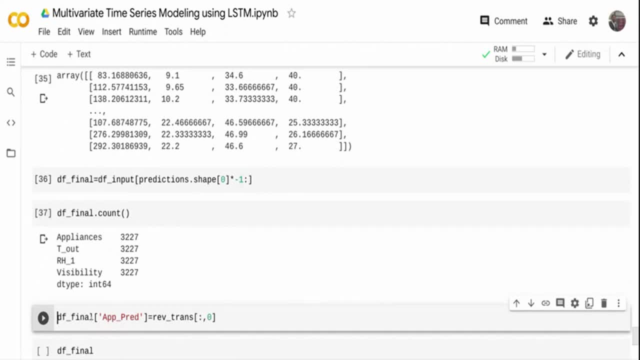 Right now, what I'm going to do is I am going to create one more column, the DF final, which is the appliance usage predicted value, And in the reverse, the reverse transformation that I did on the top. I am just going to pick the first column over here. 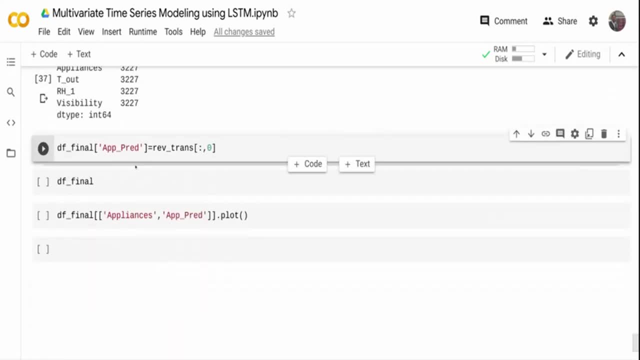 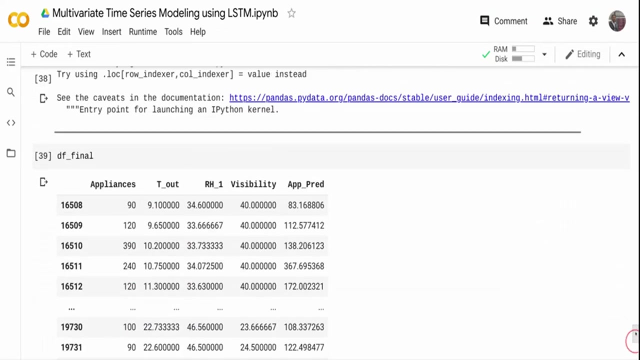 That is the predicted appliance value. So that's what I'm doing over here. I am creating this. taking this predicted appliance value, I am attaching to the DF final data frame, which is the operator. Now, if you see the output over here, I will basically have this over this. 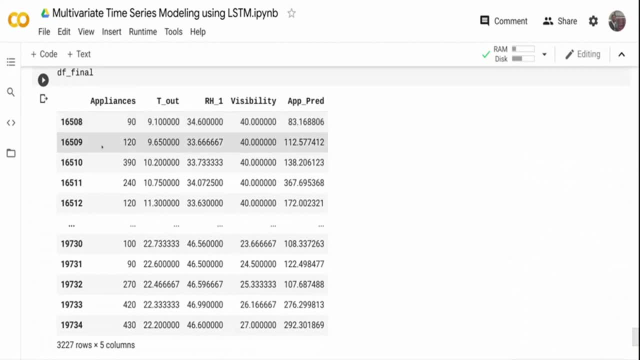 So this is the appliance: actual value: 90.. The predicted value is 83, 120.. The predicted value is 112, 390.. The predicted value is 138, 240, 367.. So, basically, this is how it looks like.